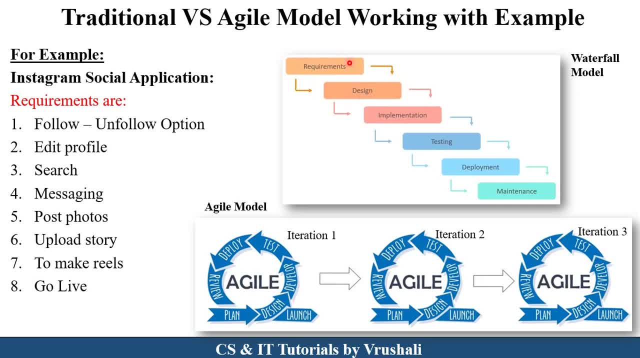 Now, what is the concept of waterfall model? First, they gather all the requirements from the customer, So there are total eight requirements from the customer. For example, now they design the product, implement the product, testing the product and after completing this product, they deploy to the customer and at the end they take a feedback from the customers. right, This is a concept of waterfall model. Now suppose we use agile model for development purpose. See here, What is a concept of waterfall model? 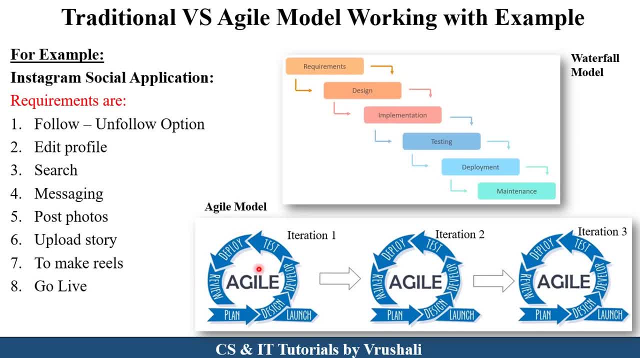 What is a concept or working of agile model? In agile model the first is requirement gathering. They collect all the requirements from the customer and they ask highest and priority wise requirements. Suppose customer want first three requirements that has highest priority, like follow and follow option, editing profile and searching. So in agile model in first iteration they develop these three requirements first. They design, develop and test these three requirements first. 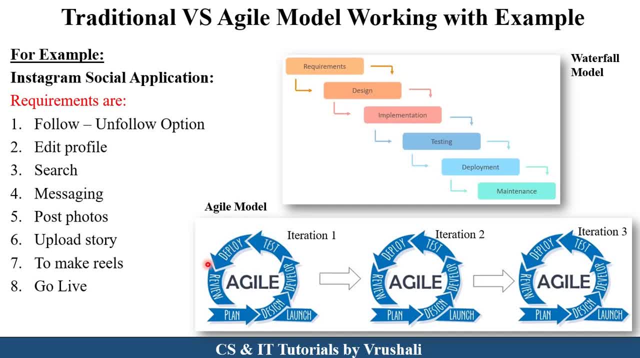 As a product: okay, and they deploy it to the customer. Now they take a review or feedback from the customer according to this three requirement development. If customer want any changes, they move to next iteration. Okay, in this next iteration they made a changes as per the customer requirement and they develop next three requirement like searching, messaging and post photos in next iteration. Okay means they design, develop and test these three requirements. 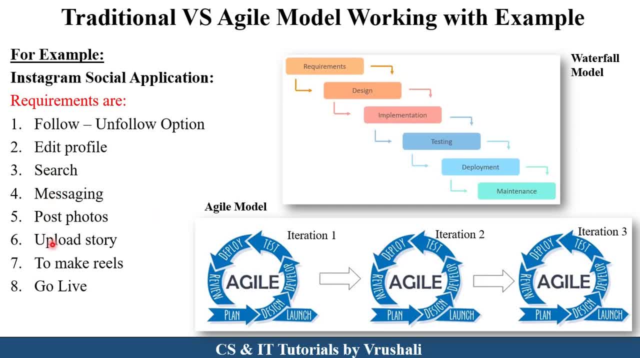 Develop, test, deploy these three requirements. Okay, Now after deploying they again take a customer feedback. If customer want any changes, they move to next iteration and next iteration they solve those changes and again develop next two requirement. like to make a reels and go live this kind of requirements. Now they design, develop, test and deploy this requirement. So at that time this all happens. 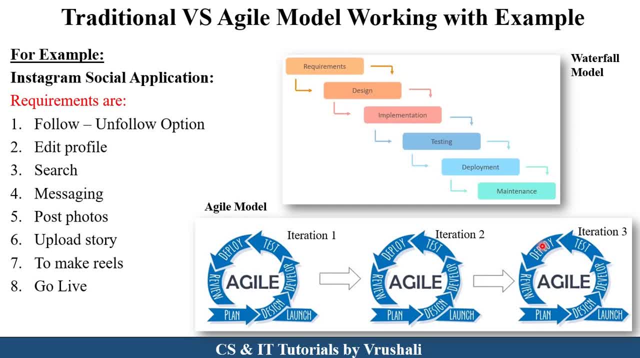 All requirements have fulfilled Then they deploy it to the customer and again take a customer review. If customer want any changes, they solve all these changes and again launch the product. So this is a working of agile model. Agile model divide complete requirements into the multiple iterations and they developed a product as per the priority of the requirements. Next now see here Here traditional. 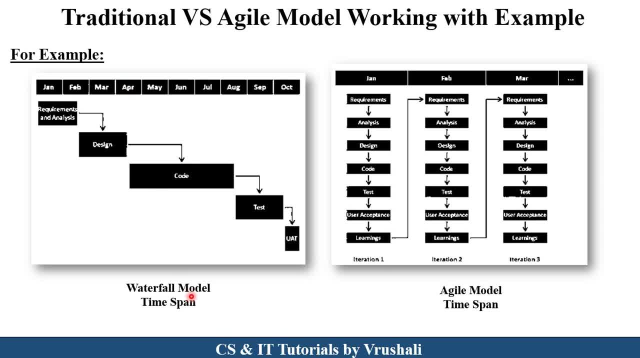 waterfall model required, how much time for development and how much time required for agile model. for development, Suppose in waterfall model, it take a two months for requirement gathering and analysis phase, Okay. After that it take almost one and half month for designing purpose And after that they almost take a four month for coding purpose and one and half month for testing purpose And at the end if any changes want required customer for that one purpose, we almost they required. 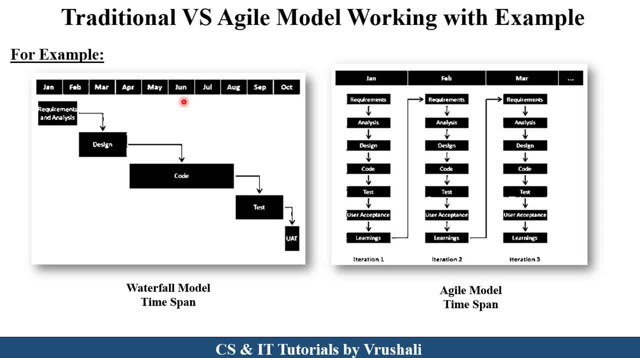 development purpose almost eight to nine months Right. But now in agile model in first iteration they take almost three to four week for development purpose. Now, after developing first iteration, they move to second iteration for three to four week and again move to next iteration for three to four weeks. Right Means for development purpose they required only three months. So that's why agile model used in each and every software nowadays. Agile model required. 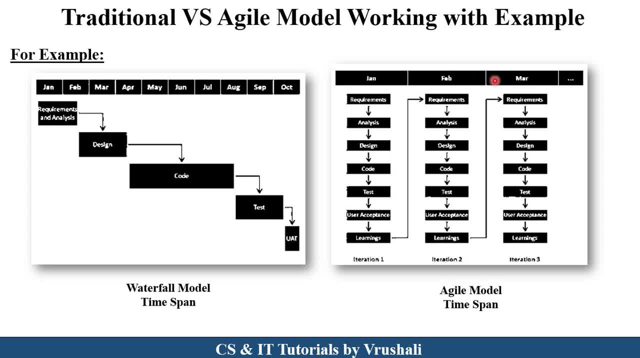 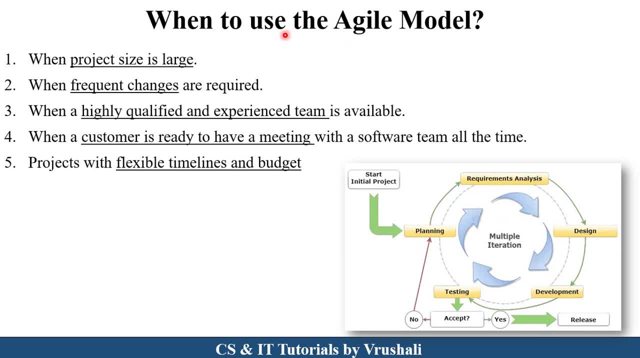 minimum time for development, with greater accuracy and greater quality of the product Clear. Next. Now the important thing is when to use agile model. See when your project size is large and ongoing project and when continuously changing requirements, your requirements are not fake. Customer interaction is more. For developing agile model, you have to require highly qualified and experienced team. 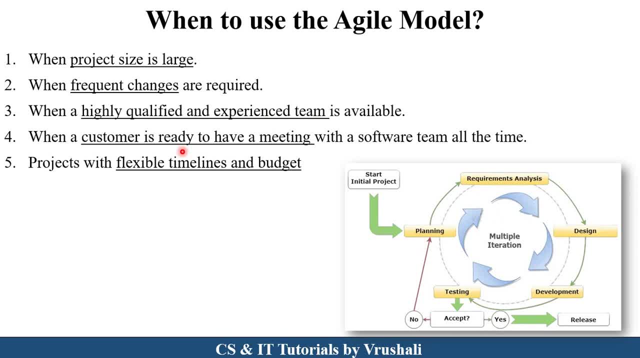 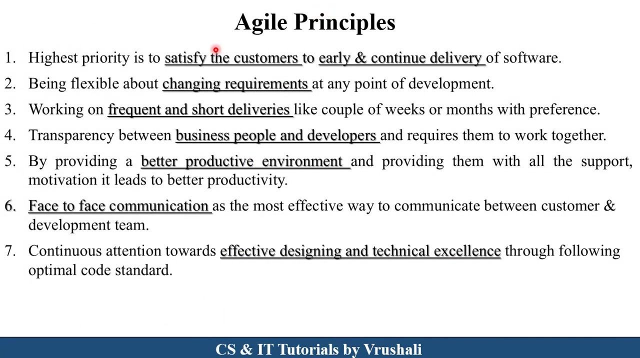 And here, after every iteration, customer interaction is there. Right Means here. customer is ready to have a meeting with software team all the time after each and every iteration And this project with flexible timeline and budget, there is a rapidly development of the product. On this phase, agile model have used. Now there are different agile principles. Agile model follow total 12 principles. That's why agile model is used. 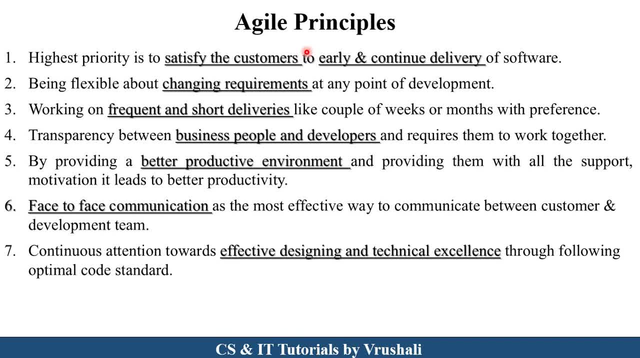 Agile model have used in different software product. nowadays The first principle is to satisfy the customers in early, continue delivery. The first important principle is here: in agile model The highest priority is customer interaction and customer feedback. After each and every interaction they take a customer feedback and there is a early and continue delivery of the software. In two week they deploy first. iteration means first three requirement of the product. 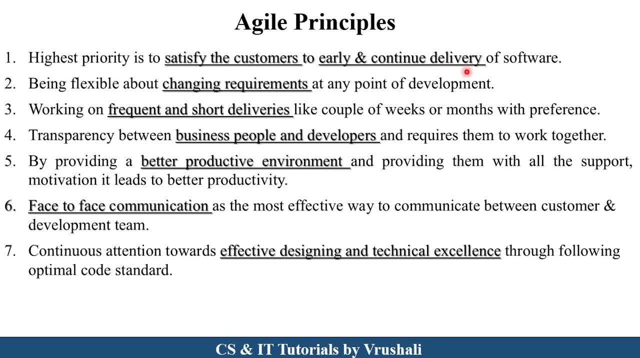 Of the particular product. After that they deliver next requirement And after that they deliver next requirement. in this way Mistake early and continue delivery of the software. The next principle is changing requirements. Here customer can change the requirements in any phase. Right, That's why it is flexible for the customer and customer satisfaction is there. The next principle is frequent and short delivery means each and every iteration They deployed. 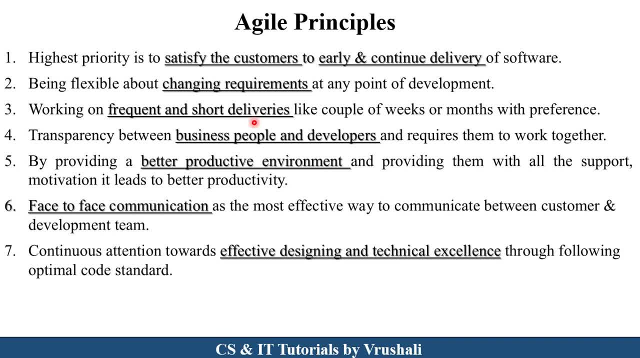 to the customer after couple of weeks or couple of months, Right. The next principle is for transparency between business people and developer. Here every stack holder means customers requirement gathering than project head, developer tester. Everyone work together. This is a main advantage of agile principle. That's why there is a better productive environment And due to this better productive environment and all the stakeholders. 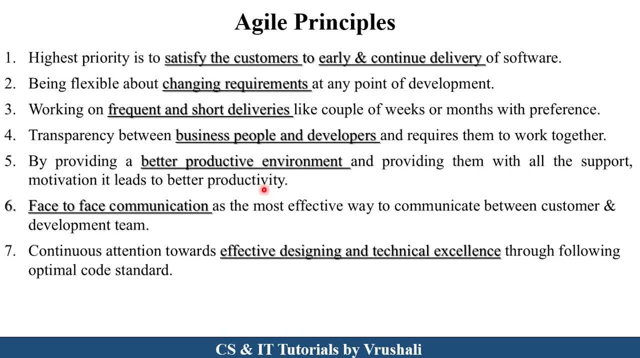 can work together. that's why it leads to better productivity and better quality of the product. The next principle is face to face communication. Here, after every iteration they take a customer feedback means there is a face to face communication between customer and development team. That's why. 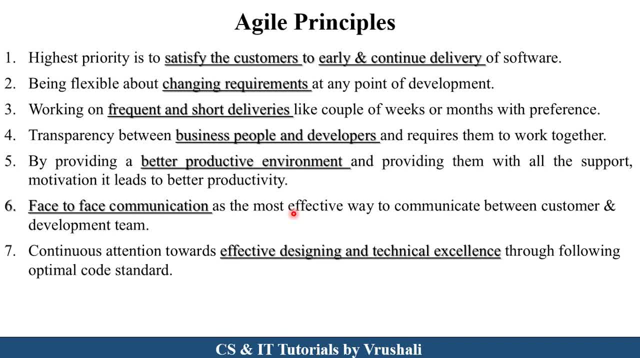 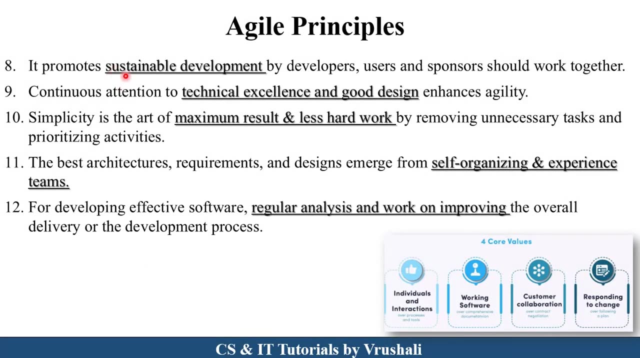 there is the accuracy of the product and customer satisfaction. The next principle is effective designing and technical excellence. due to involvement of the customers, They design accurate of the product and more time they do on the implementation of the product. they follow proper coding standards and different designing standards. now the next principle is sustainable. 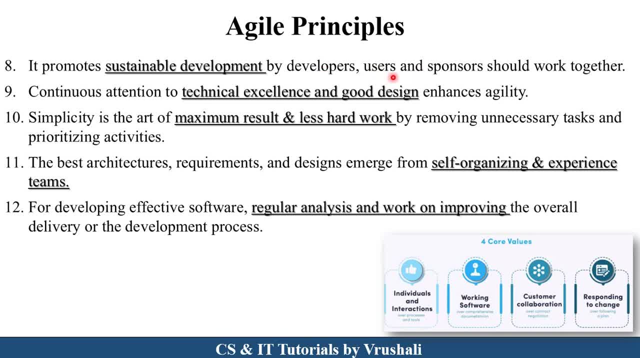 development. here all the developers, users, sponsors, all are work together and there is a rapid delivery of the product. that's why it promotes the sustainable development. and next principle is there is a continuous attention on technical excellence and good design. if there are good design, is there then only developer develop a product more accurate way. right, the next agile. 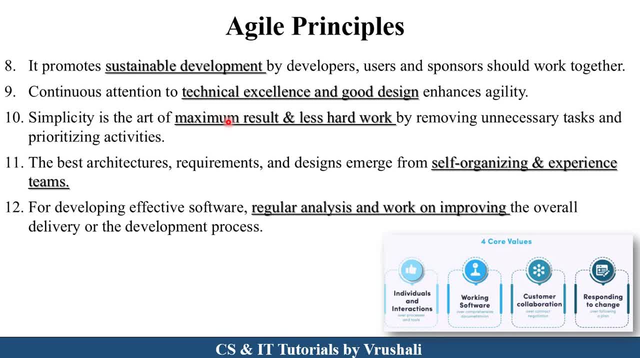 principle is simplicity here, maximum result and less hard work. in agile model they can't waste time more on requirement gathering on planning phase. they required more time on designing and coding part right. that's why there is a maximum result and less hard work. no documentation: work is there or less documentation. is there right? the next agile? 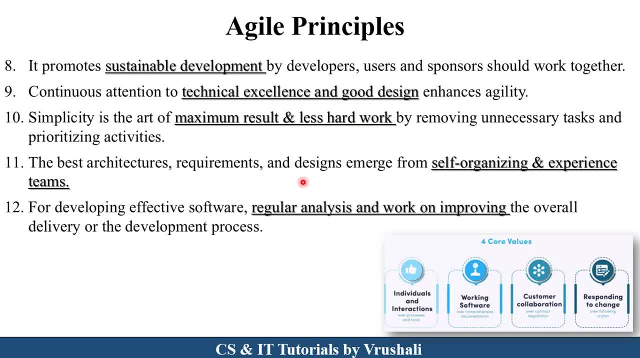 principle is self-organizing and experience team. as we discuss for developing agile model, it required highly qualified and experienced team because there is a rapid development and customer satisfaction is there right? and last one is regular analysis and work on improving. after every iteration they take a customer feedback, so it is very 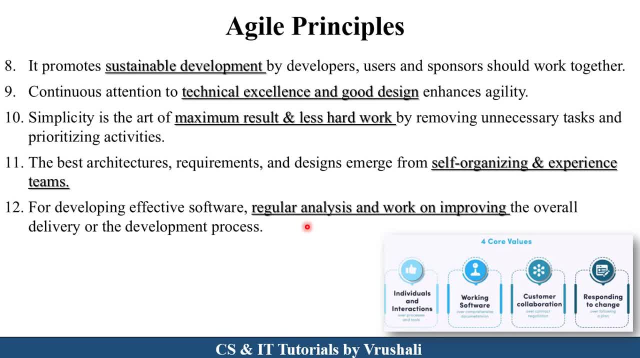 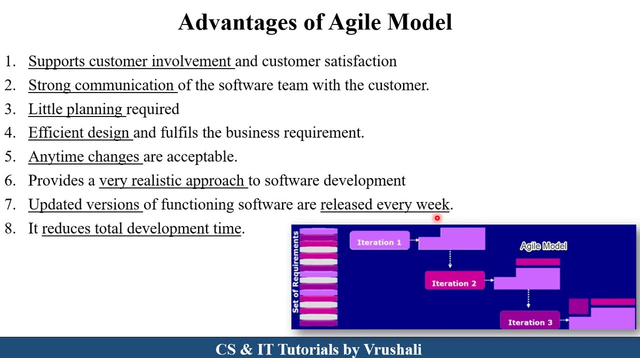 important to solve all the customer required changes and develop next iteration, next priority requirements. so that's where regular analysis and work on improving on each and every product is there. so these all 12 principles must follow in agile model development. now next one is advantages of agile model. so, as we discussed earlier, first there is a customer satisfaction and customer 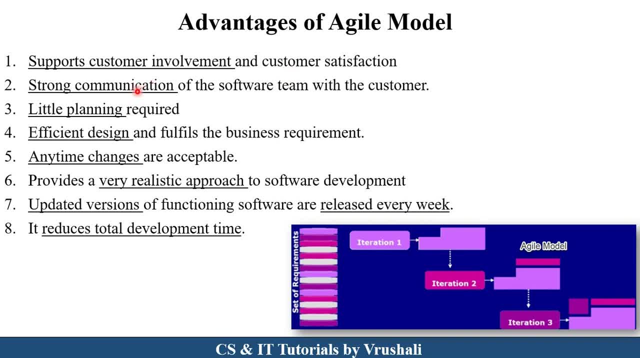 involvement addition. this is an example of agile model. in agile model design there is a strong communication between software team and customer. then there is a little planning required because they focus more on design and development phase. and in agile model there is an efficient design. they fulfill all the customer requirements and anytime changes, your requirements are continuously changes, right. 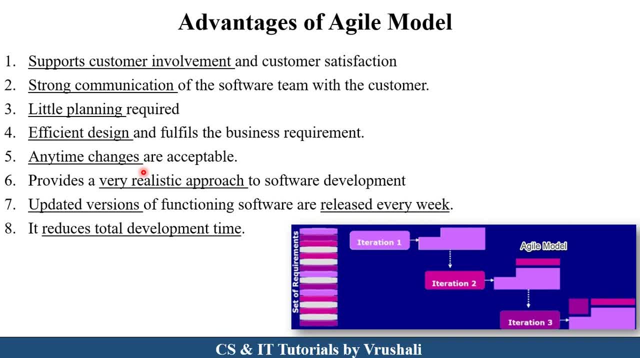 so anytime changes are acceptable in agile model. now agile model provide very realistic approach. they provide very accurate and quality of the software. now, each and every week new updates are there. in first iteration there are some new requirements. after, in second iteration there are new versions are there? let's take one example. suppose you want to buy a particular. 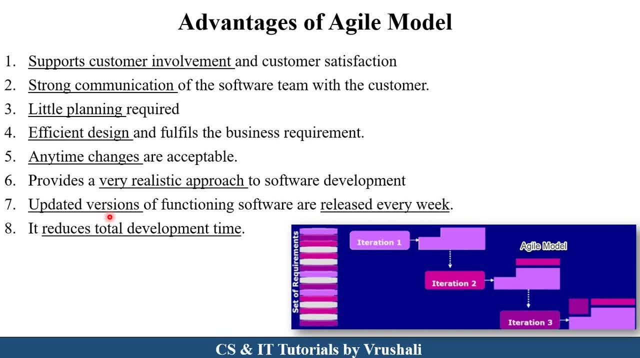 laptop, okay, and you buy this laptop in January month. suppose there is a Lenovo laptop. is there, you check all the requirements, their memory, their size, their battery, etc. right. and on next February month, again, there is a updated version of this same software, same laptop, right? so this used agile model. each and every week they release a updated version. 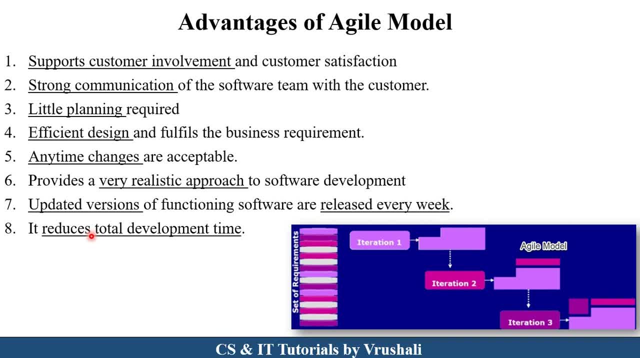 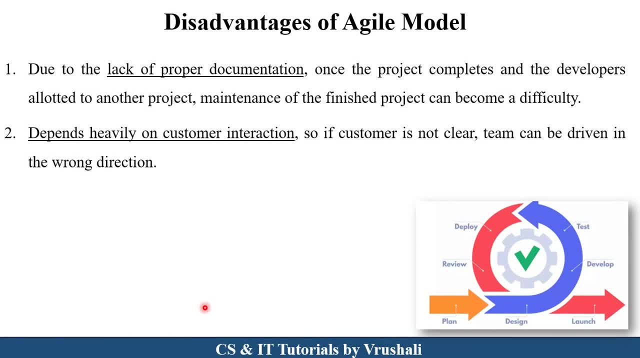 and updated features. right, and last one, is it reduced total development time? so these are the advantages of agile model. now the disadvantages of agile model. the main disadvantages is: there is lack of proper documentation. they can't waste their time on documentation and that's why there is no any proper documentation, suppose.